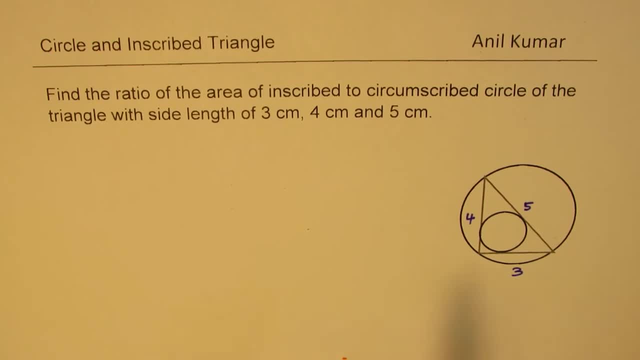 Definitely it is not. 2. We need to find area of the inscribed. that means the smaller circle to circumscribed, the bigger circle that is circumscribed. Is that clear to you? Okay, Let us see how to figure this out. 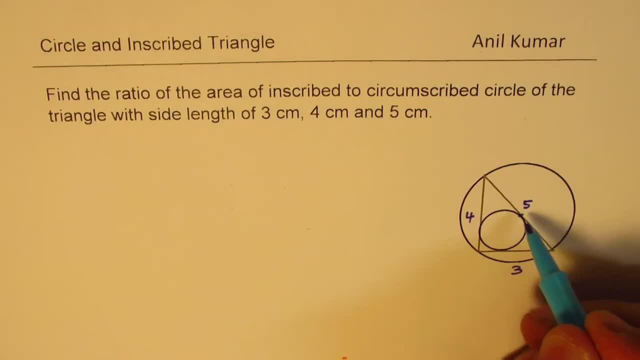 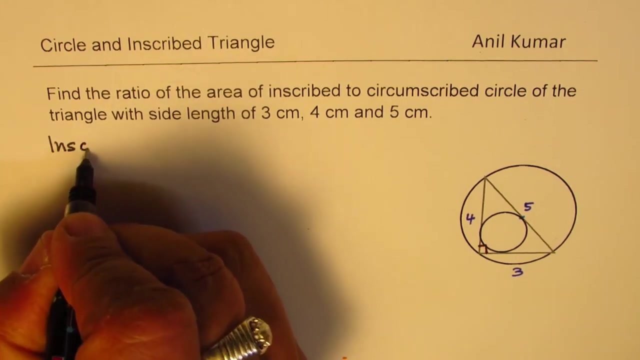 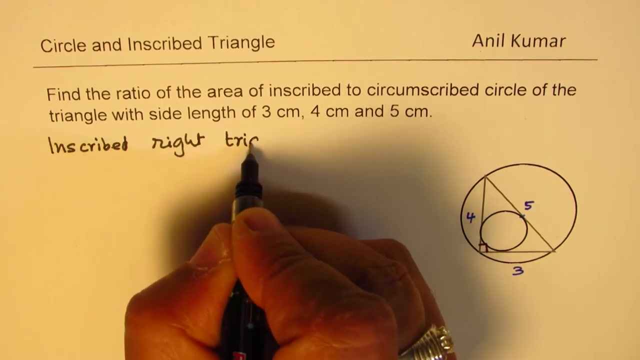 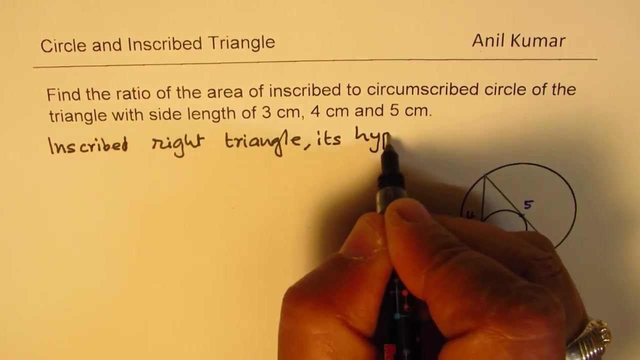 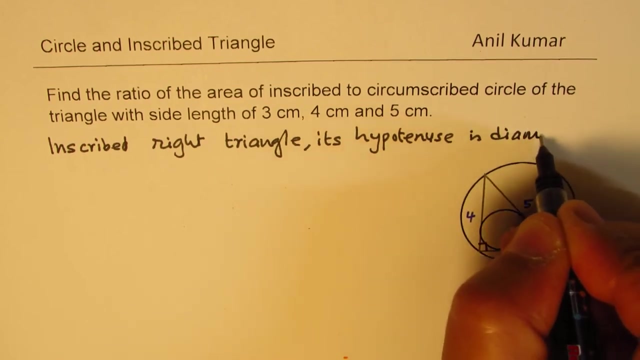 As far as the circumscribed circle is concerned, we know that this right angle triangle, which is inscribed in a circle, should be in a semicircle right. So since we have an inscribed right triangle, its hypotenuse is diameter of the circle Clear. So since the circumscribed circle is in a semicircle right, So since the circumscribed circle is in a semicircle right, Since the circumscribed circle is in a semicircle right, So 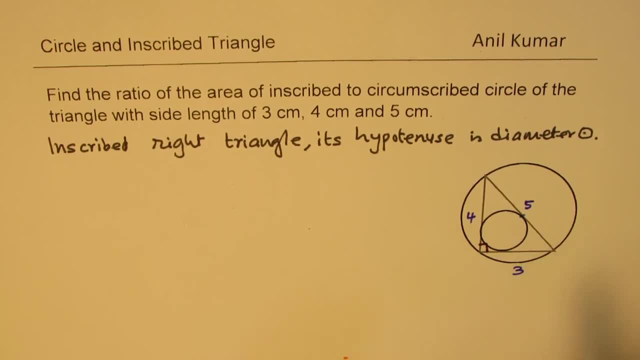 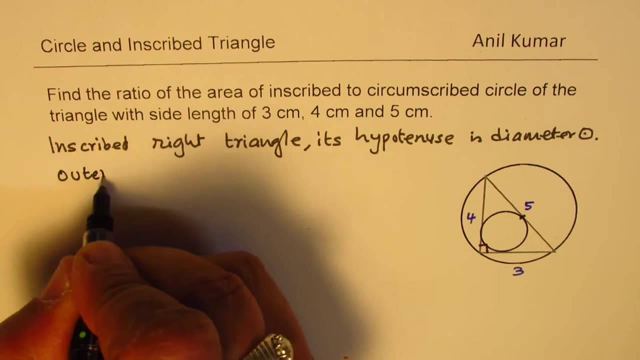 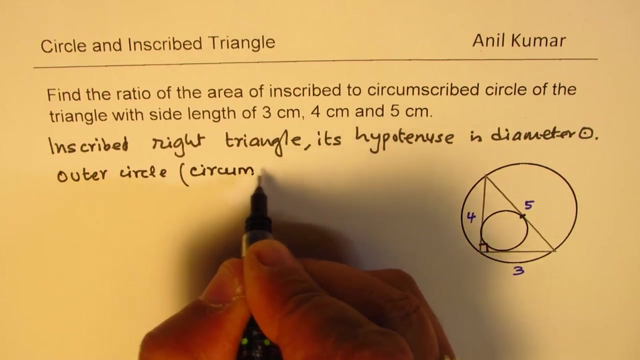 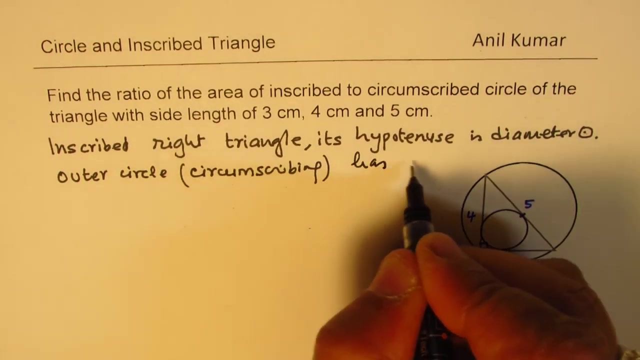 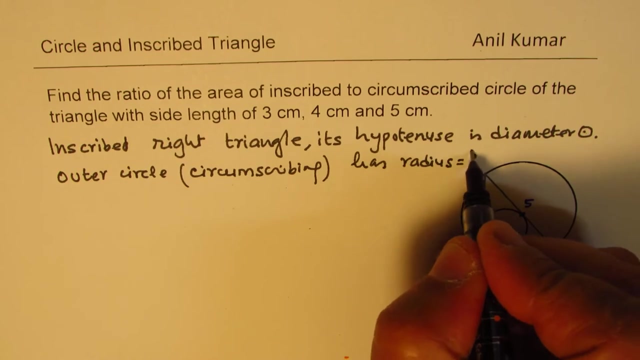 this is 90 degrees. that has to be the diameter of the circle. So if it is the diameter, that means outer circle, we mean circumscribed circle- has radius equals to 5 by 2.. Right, 5 is the side half of the diameter currently. 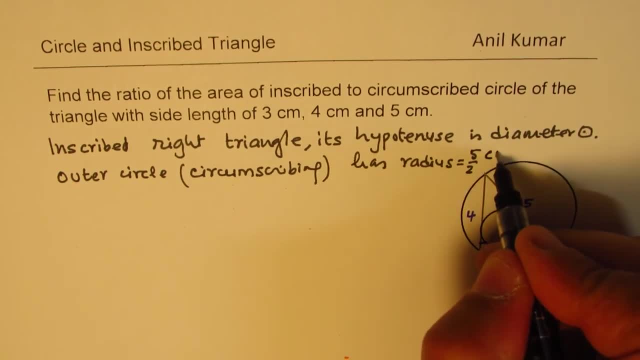 So those many units, let me write centimeters, half of five. now the question is: how do we figure out the radius of the smaller circle? now, this is a very important technique which you will see, helps in solving many questions. so look here at the diagram very carefully. 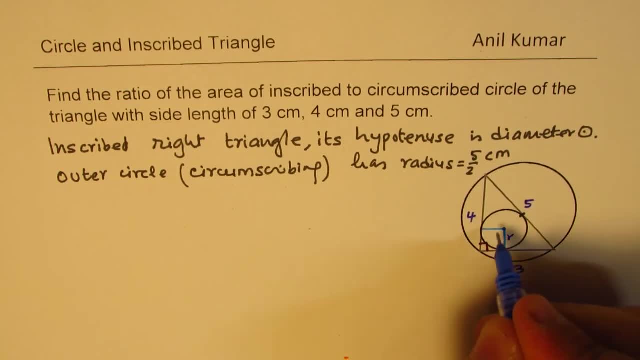 that is the radius right. so what do we notice here? we notice that this circle which is inscribed touches the triangle right. therefore, this side which we have here will be this: is r 3 minus r. so if you look from this vertex, we have a tangent and another tangent, so two tangents. 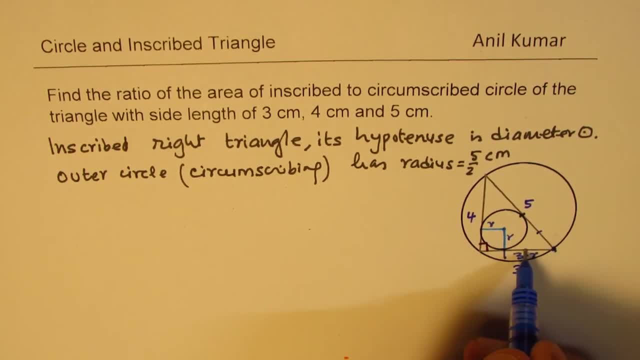 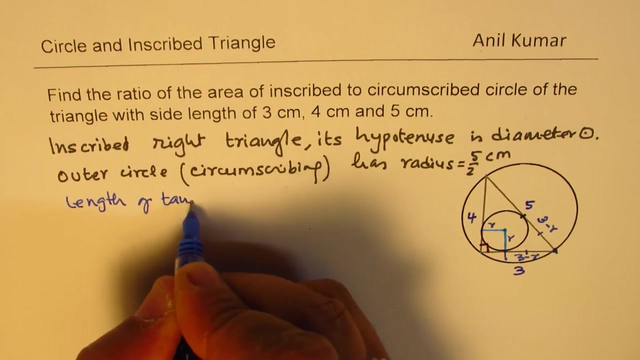 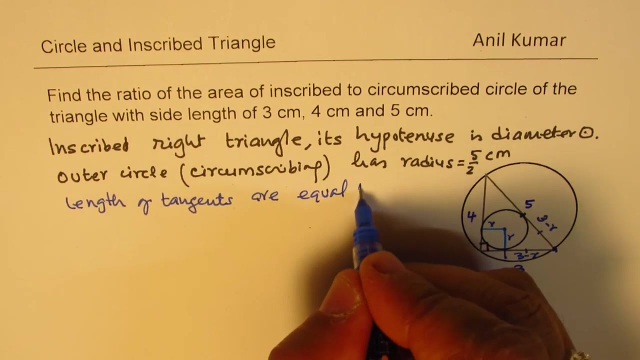 so that means that the tangents should be equal, right? so this side is also 3 minus R. is that clear? so important properties to use here is that the length of the tangents are equal from a point. is it clear to you, right? so so from this particular 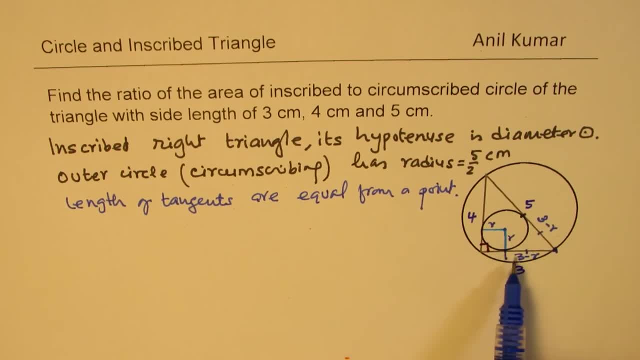 point. both the lengths are equal and we found that since the circle of radius, small r is inscribed, the length should be 3 minus R, whichever I have written here right. similarly, the the other length is 4 minus R, so this will be 4 minus R, since 4 less than all right. so so this length will be equal to the. 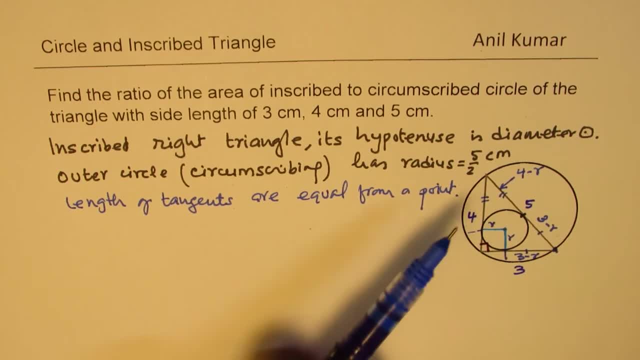 other length, which is 4 minus R. now you can see that the high port in use actually is 5 units. since it is 5 units, we can say that 3 minus R plus 4 minus R is equal to 5. okay, so whenever you have this kind of a situation, you can see that the perimeter is kind of 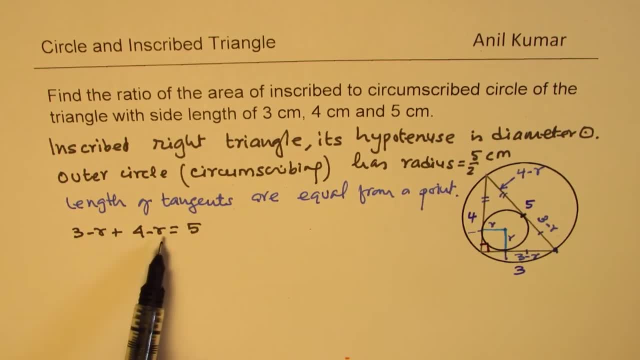 related. right, okay, we can find the value of R from here, so to our will take it on this side. so we get 3 plus 4 minus 5 equals to 2 R. now that is also a standard formula which you can always use. so you can see 2 legs minus the high potency divided by 2. is it clear to you? 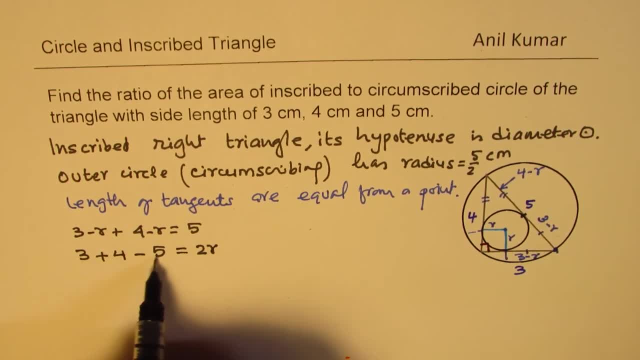 right? so which is 7 minus 5, right? so let me rewrite this: R is 3 plus 4 minus 5 divided by it. so this is a standard formula. if you have a right triangle inscribed in a circle, then you see that the length of the tangents is equal to. 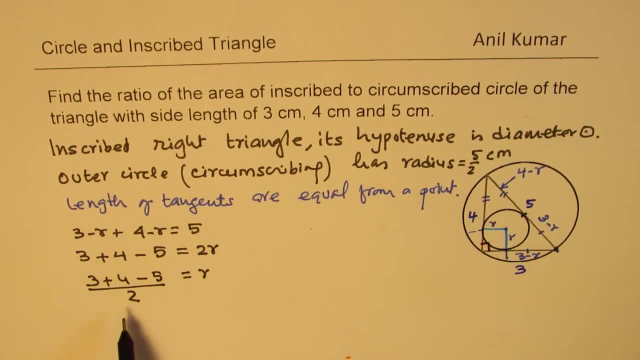 this side, sum of two sides minus the hypotenuse, divided by 2, gives you the radius of inscribed circle. perfect, so, which is definitely equal to 7 minus 5 is 2. divided by 2 is 1 unit, so the radius of this circle is just 1 units.